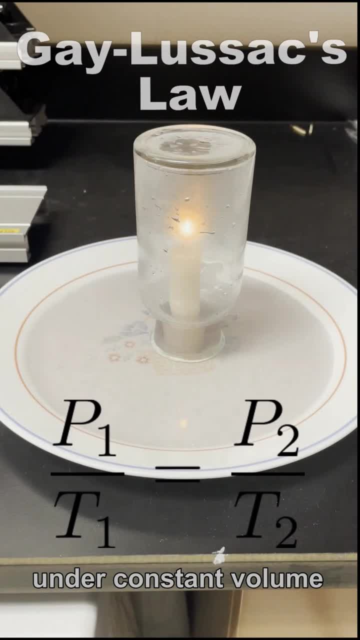 is directly proportional to pressure under constant volume, And these three laws can come together to give us our answer. Combined gas law formula.